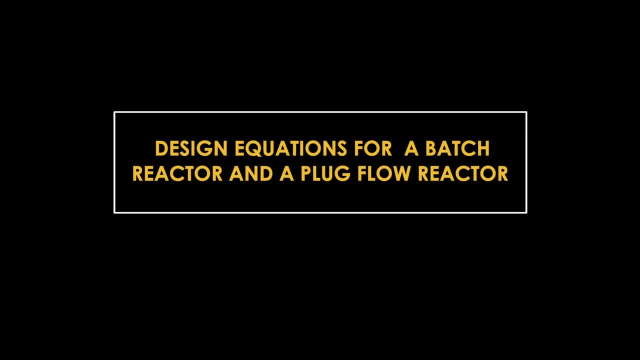 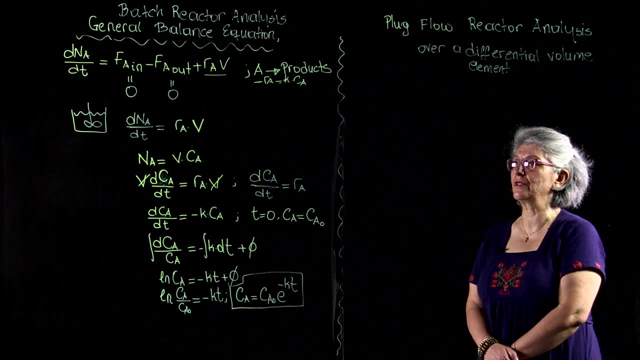 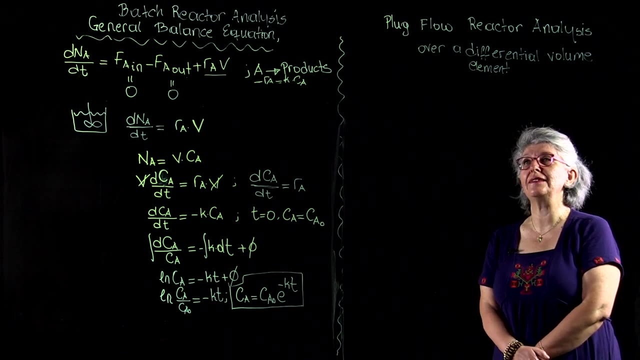 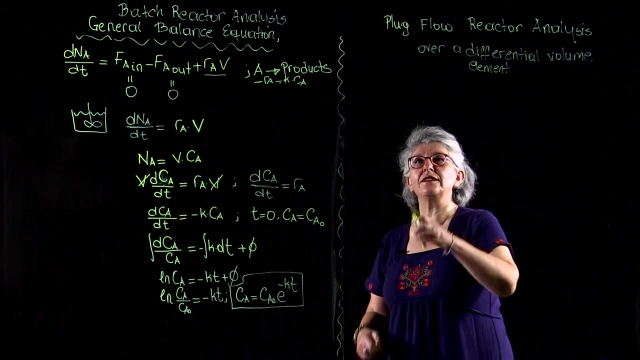 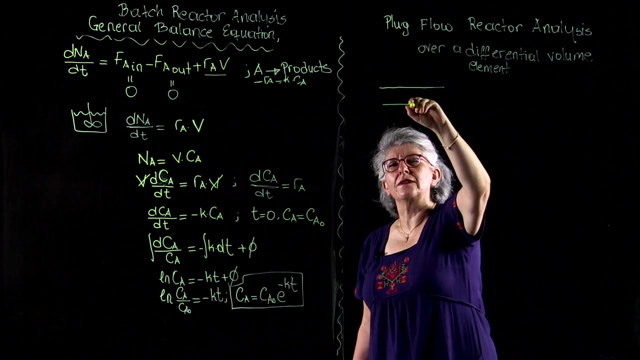 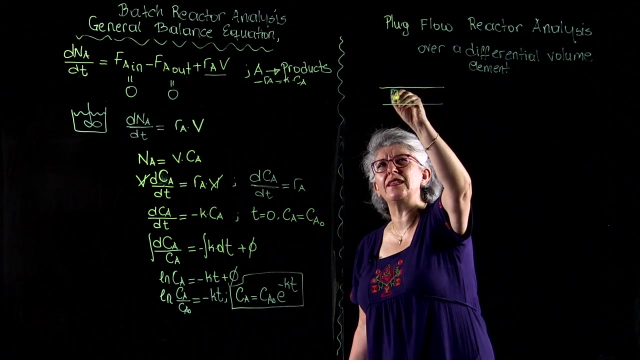 In this recording we will continue our conceptual development of the different types of reactors and their behavior, And here we will derive the design equation for a plug flow reactor which, as we learned so far, is a tubular reactor where the fluid element is moving like a plug. 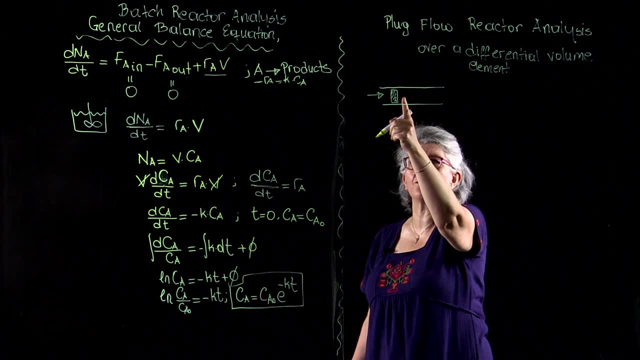 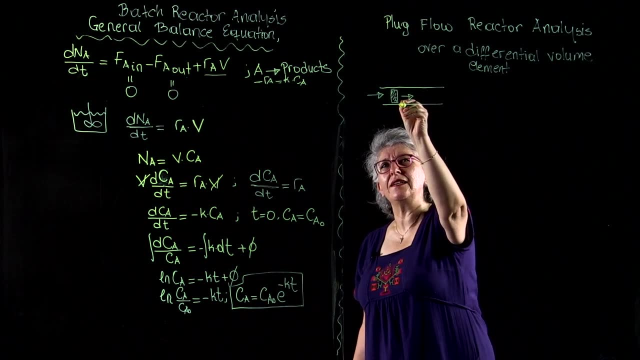 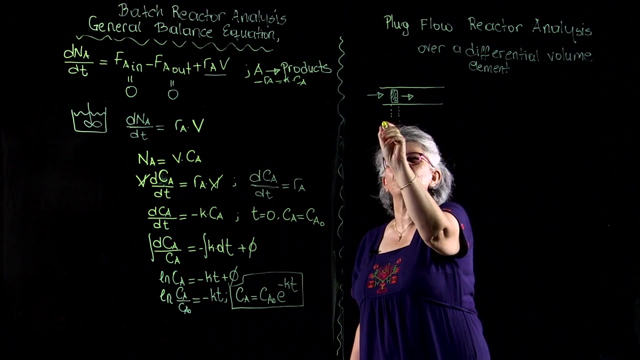 In other words, it's not mixing with the fluid element in front of it, nor it is mixing with the fluid element behind it. So here I'm going to define a plug flow reactor. I'm going to define a volume element which is going to start at z and it is going to end at z plus delta z. 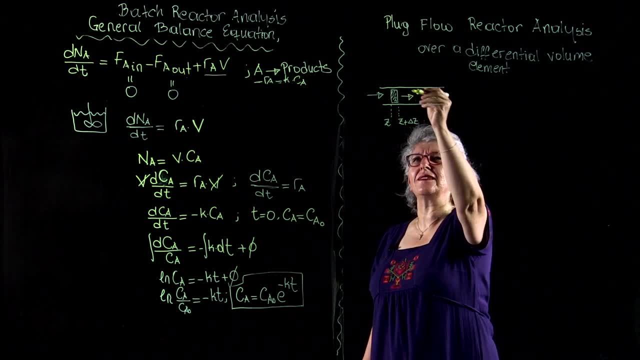 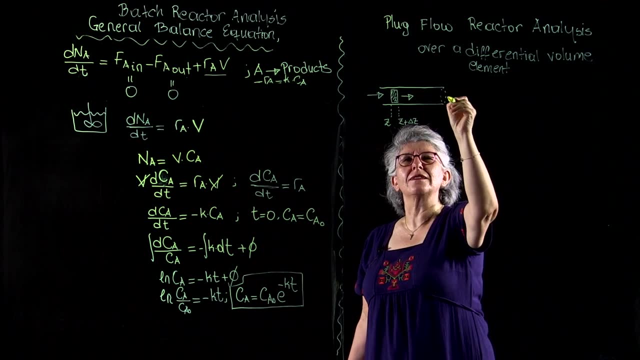 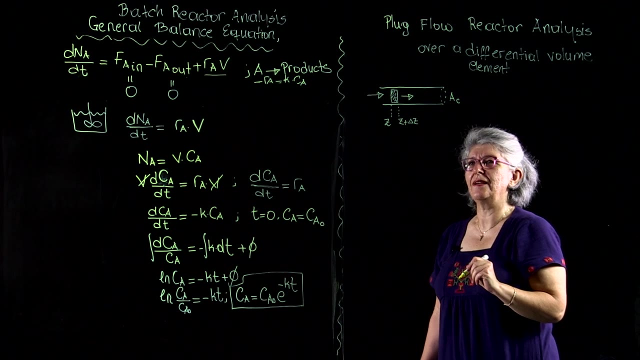 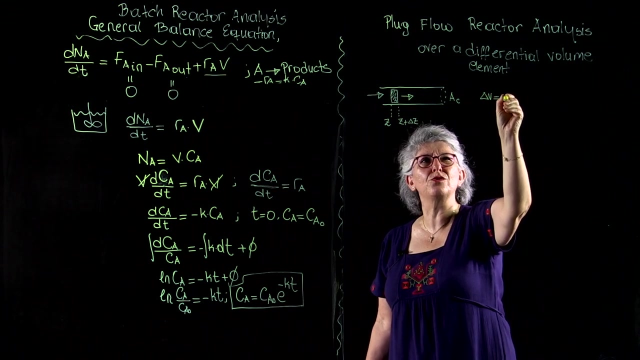 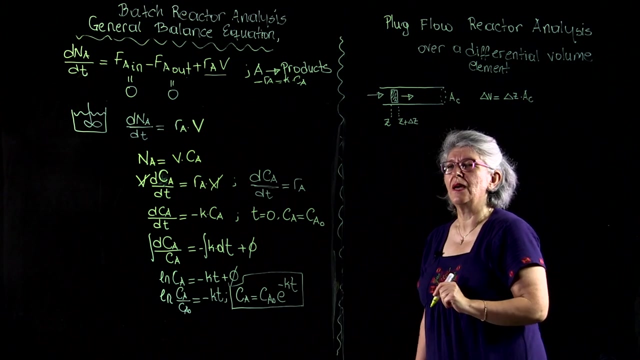 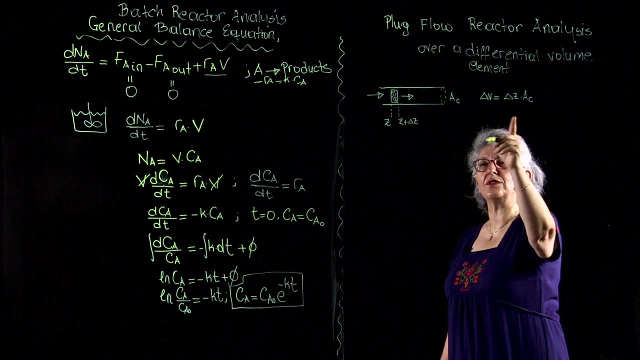 And this is going to be a cylindrical geometry. The cross-sectional area of this system is going to be A sub c. Alright, so my differential volume element is delta v, that is equal to delta z multiplied by A sub c. I'm going to write my balance equation, under steady state conditions, around that differential volume element. 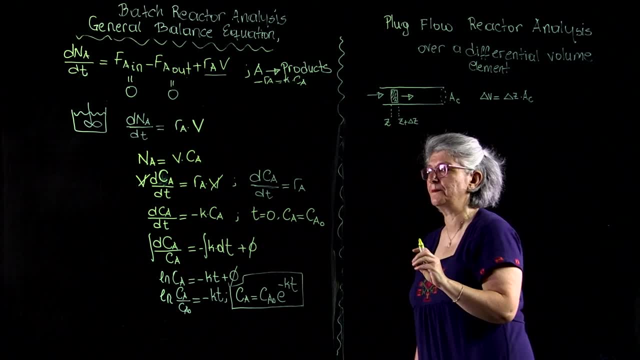 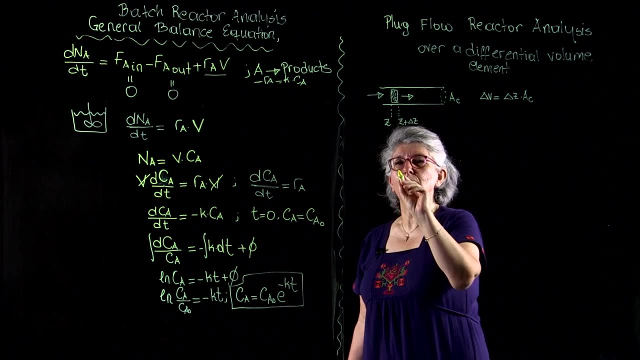 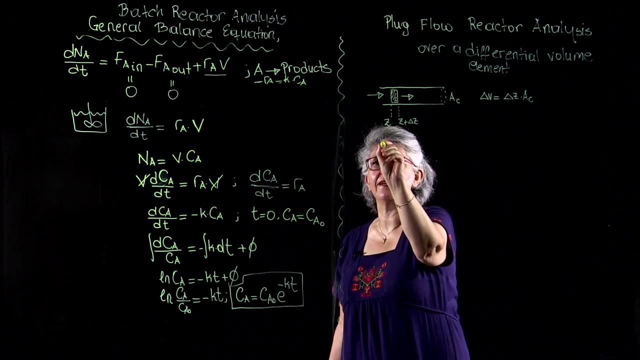 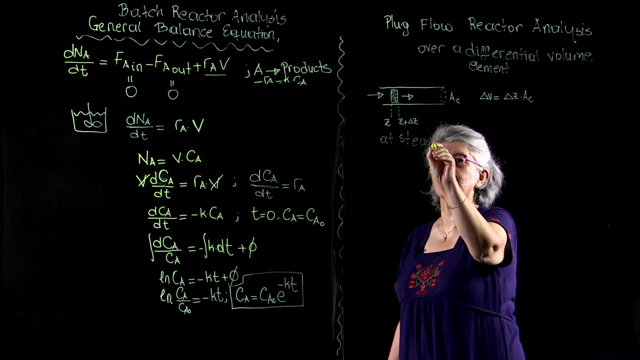 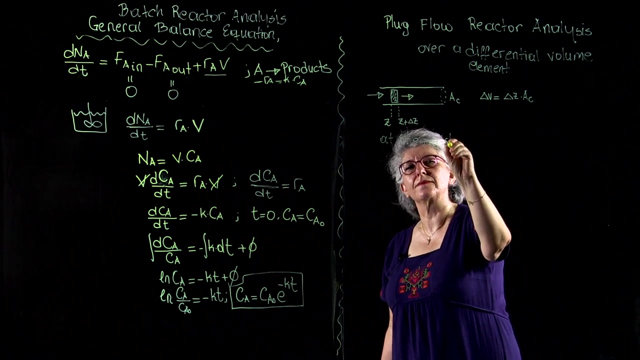 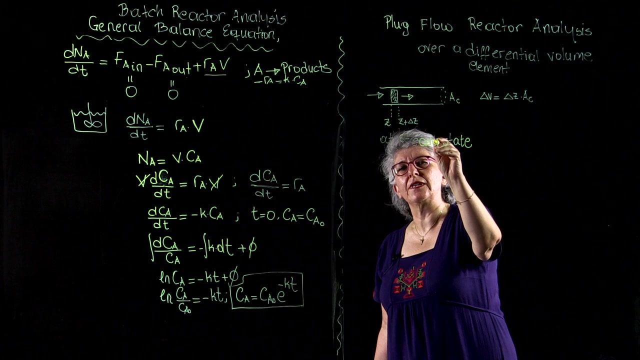 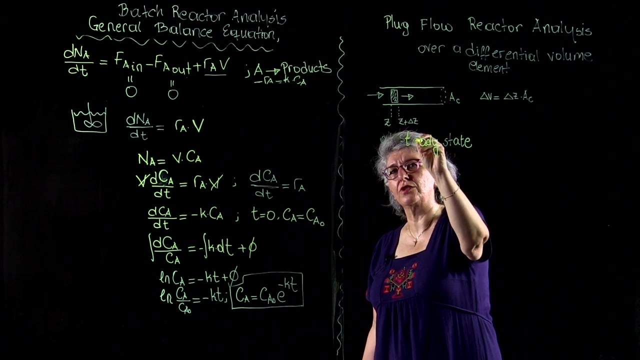 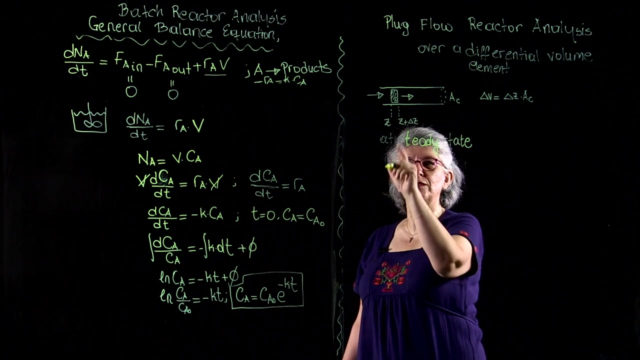 not around a macroscopic system boundary, But a microscopic differential volume element. So again, because it is steady state at steady state, right, what is steady state? Time evolution under force flows is zero. At steady state, the n over dt term is zero. 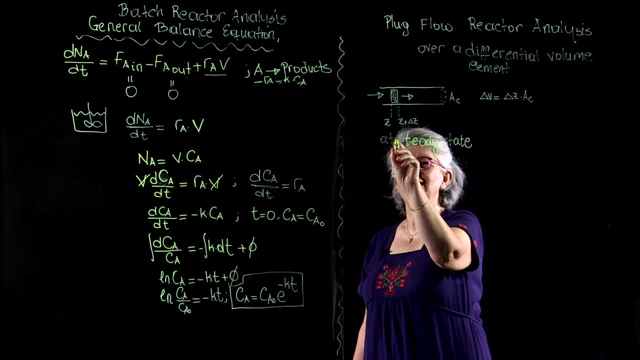 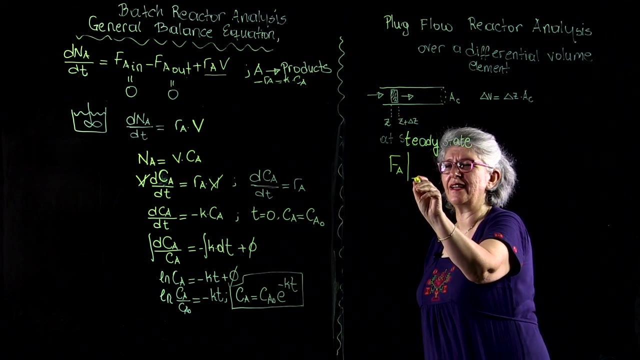 There is no time, evolution term. Then I have fluid molar fluxes F A. this time I'm writing this balance equation across this differential volume element. The entering F A is F A at z. The outgoing molar flux is F A at z plus delta z. 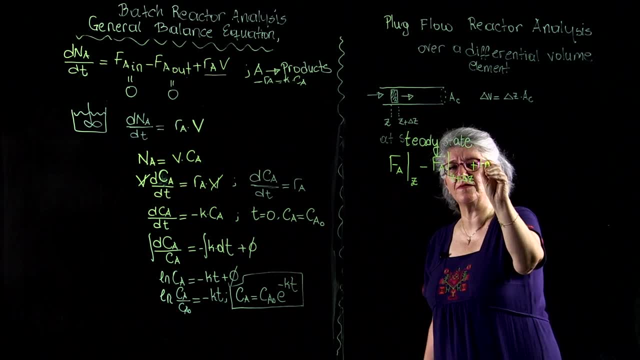 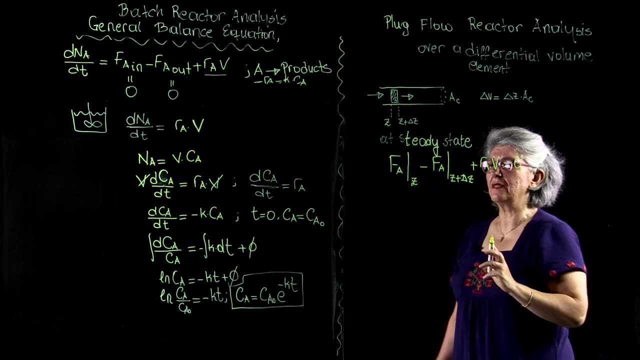 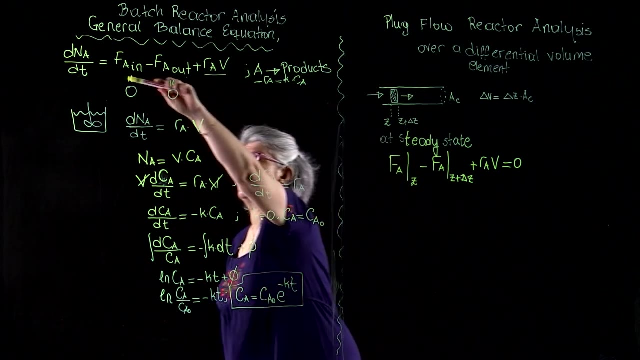 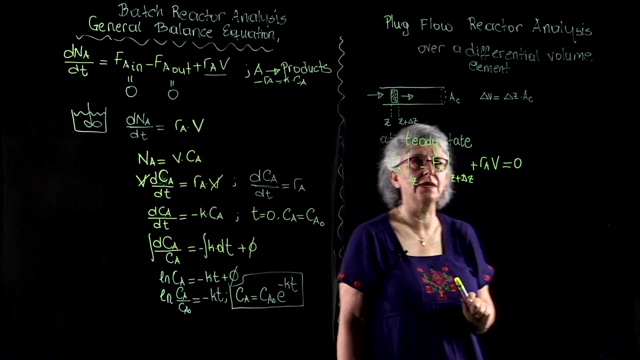 The same term. plus R, A times v, They're all equal to zero. I would like to draw your attention to the analogy between this expression and this general expression. We lost this term because our system is operating at steady state. Now this volume element. 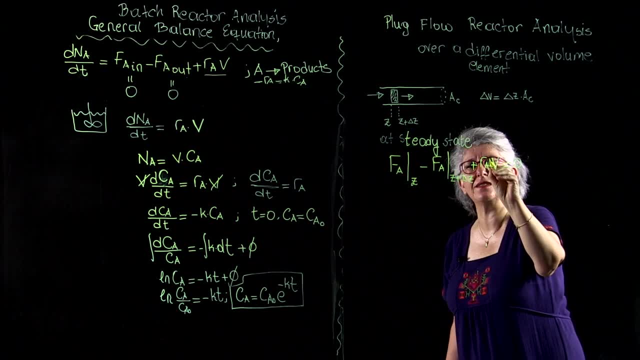 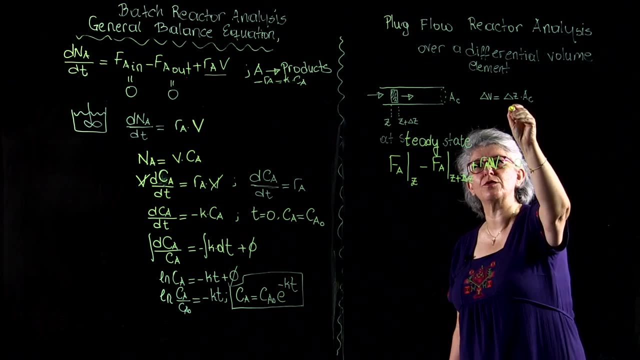 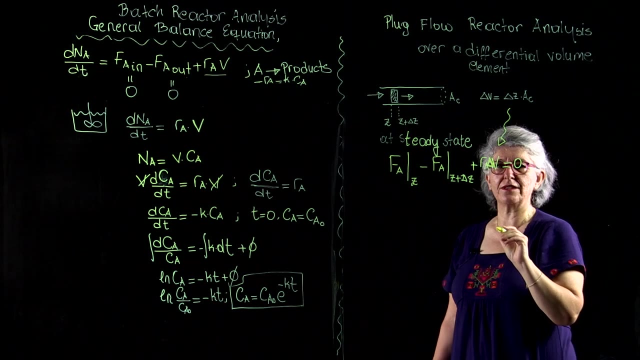 of course this is the differential volume element. right, It's not the total volume, but it is the differential volume element. I'm going to substitute this definition in here. Okay, And I will do some rearranging. First I will take these to the other side of the equation. 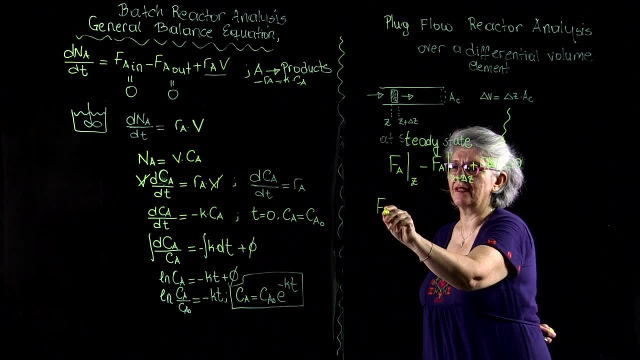 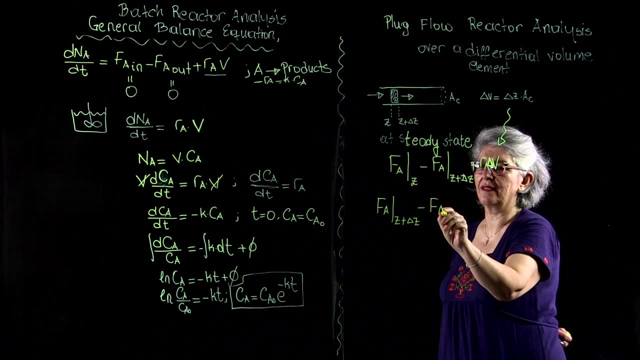 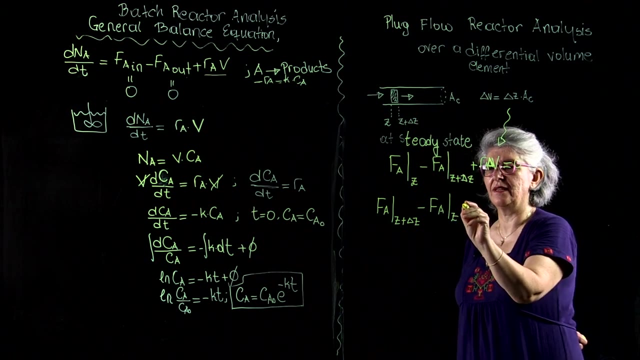 F A at z plus delta z. F A at z plus delta z minus F A at z. This is the other side of the equation. They change sign- Is equal to R A times delta v. Delta v is equal to delta z times A sub c. 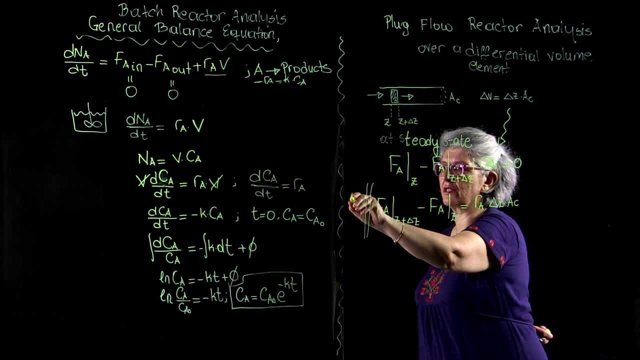 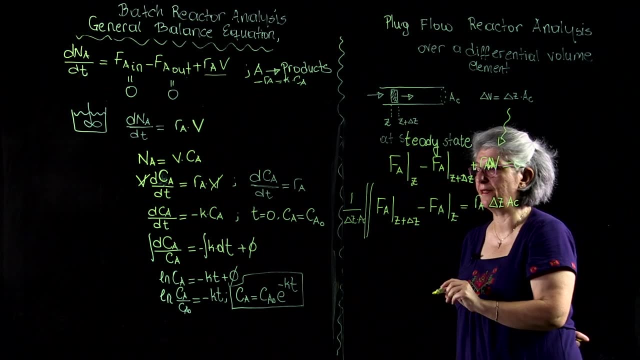 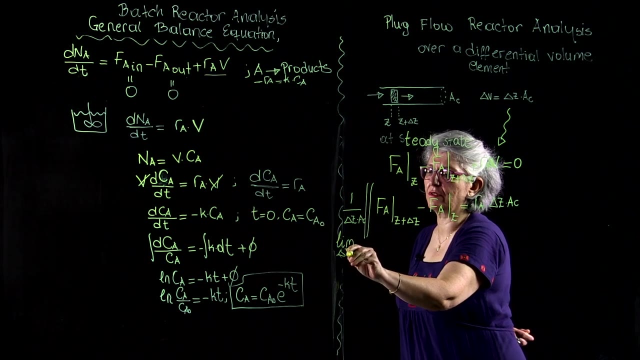 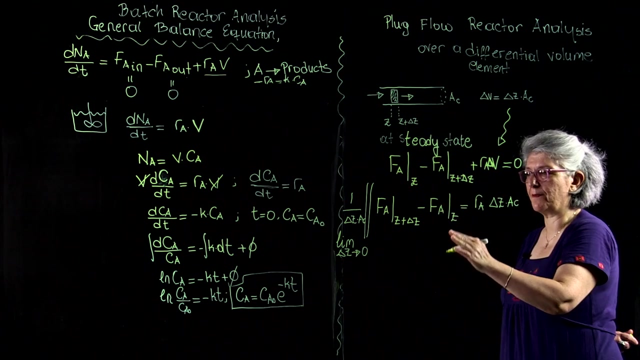 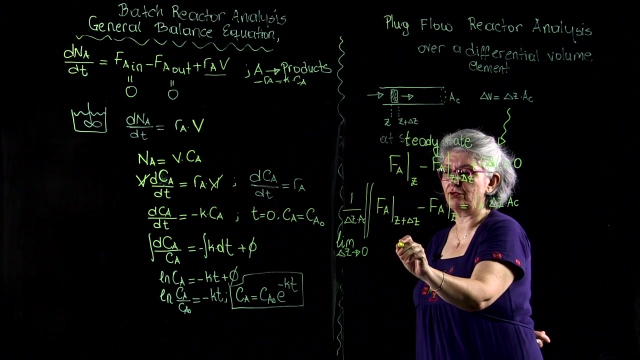 I will divide both sides of this equation by one, over delta z times A, sub c or delta v, And I will take the limit as delta z goes to zero. Okay, And as a result of this, mathematical intermediate steps that you should be able to do. 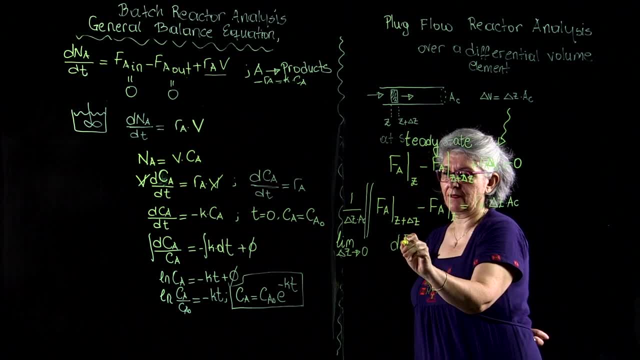 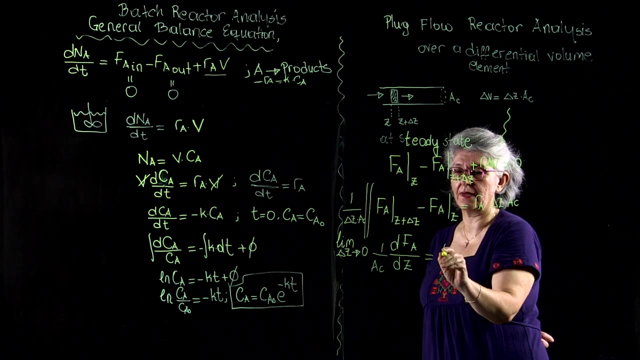 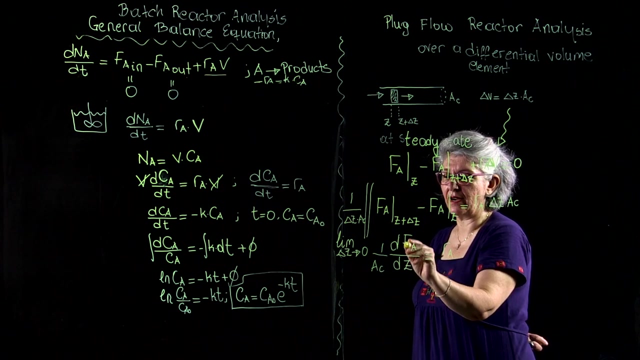 with relative ease. what I get is d F, A over d z, one over A sub c, to be equal to R sub A, Or I can combine those two terms and write this as d F, A over d, v, as R sub A. Okay. 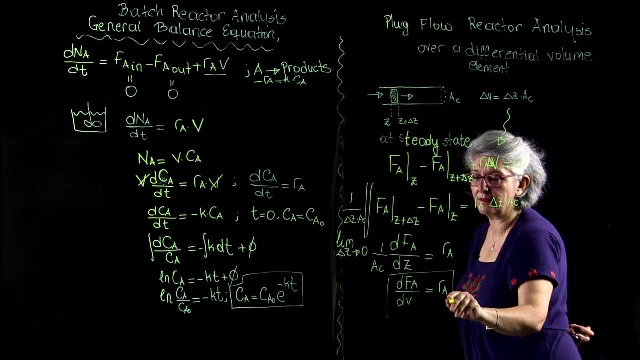 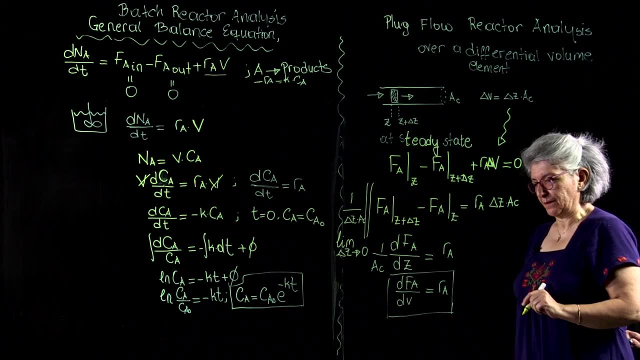 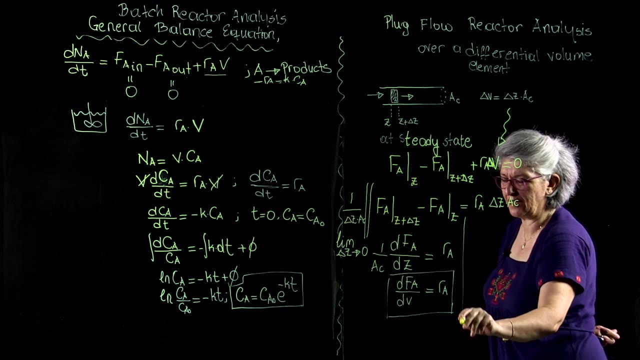 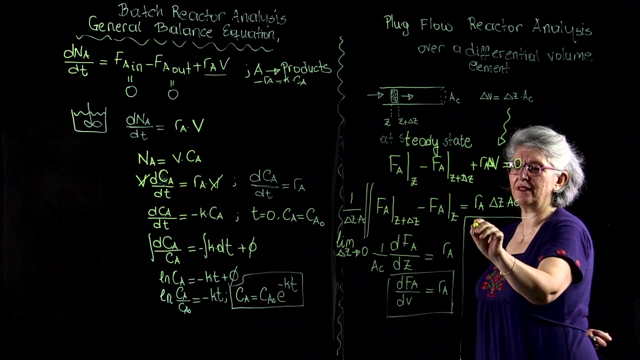 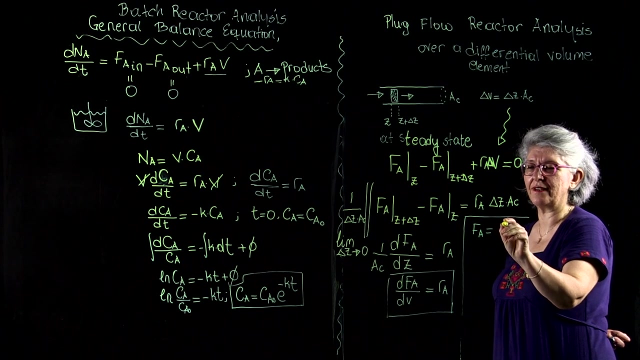 This is the design equation for a plug flow reactor. I will carry the analysis one step further Here. let me generate myself a new, clean frame. I will redefine F A in terms of its constituents. Remember F A was C A times volumetric flow rate. 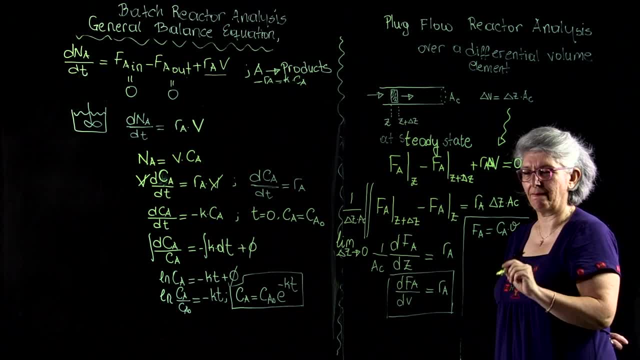 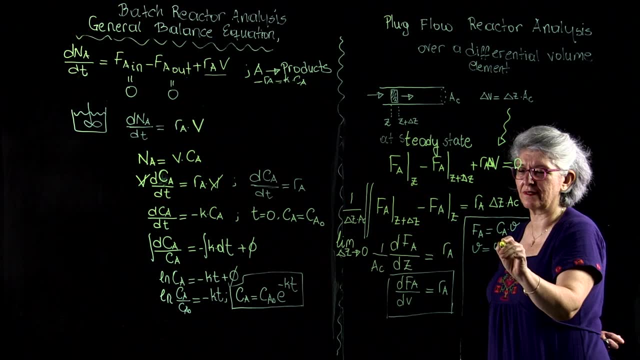 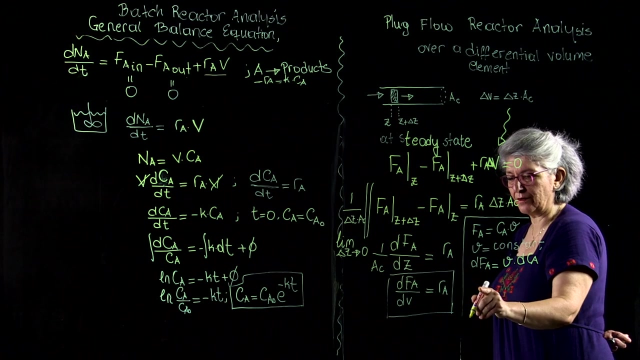 So if volumetric flow rate is constant, I can write this as d A over d z. Then my d F A can be defined as v times d C A And the design equation takes the following form: d C A over d tau to be equal to R sub A. 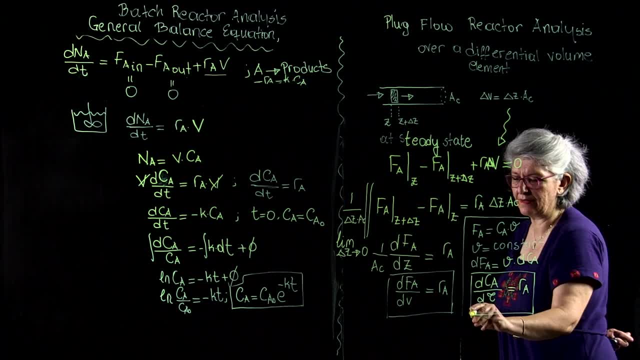 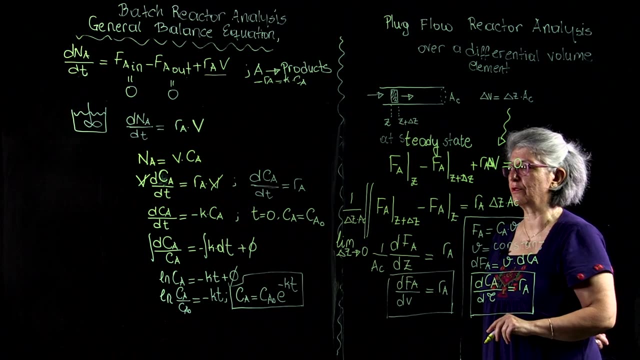 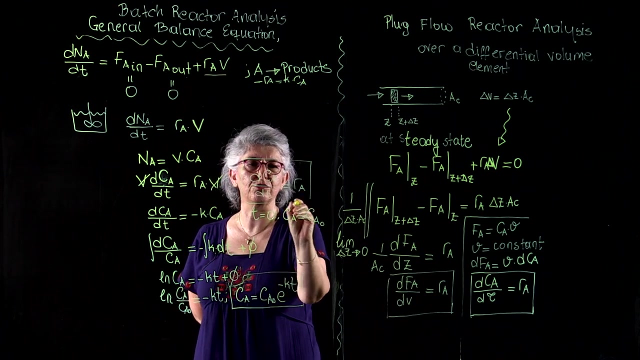 for a constant volumetric flow rate system. So I want you to compare this expression d C A over d tau to be equal to R sub A with this expression d C A over d t is equal to R sub A. This was the design equation.